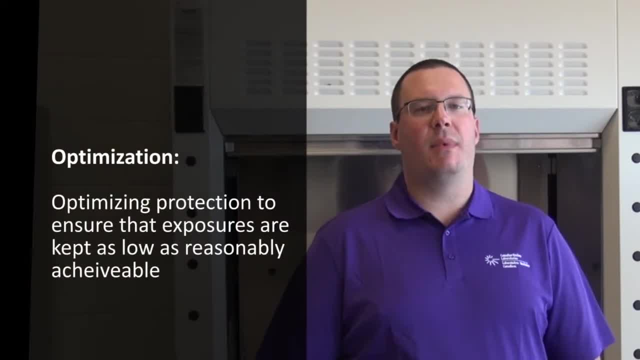 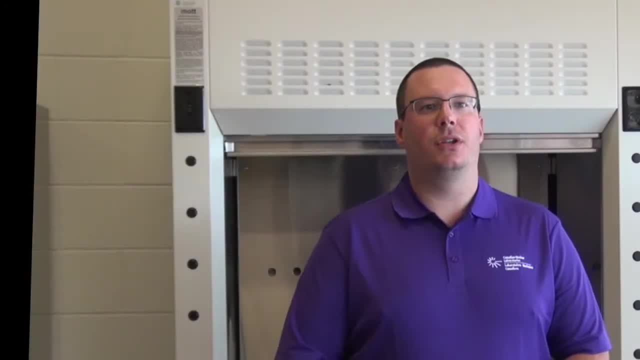 Optimization. When looking at optimization, we look at planning out a task that makes sense from all angles. It is looking at the latest information from subject matter experts and optimizing protection to make sure exposures during the work are kept as low as reasonably achievable For work. during the pandemic, this looks like gathering the latest information from health professionals to be sure that the right steps are being taken to prevent further spread of the virus. 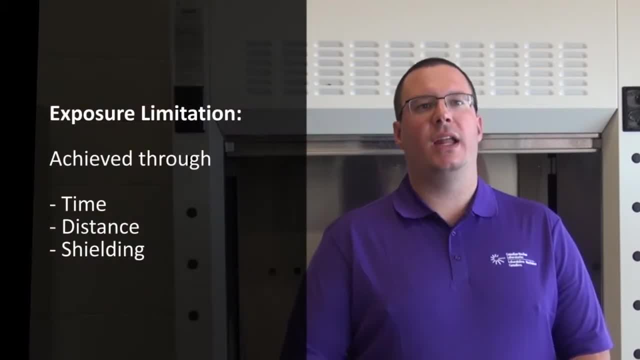 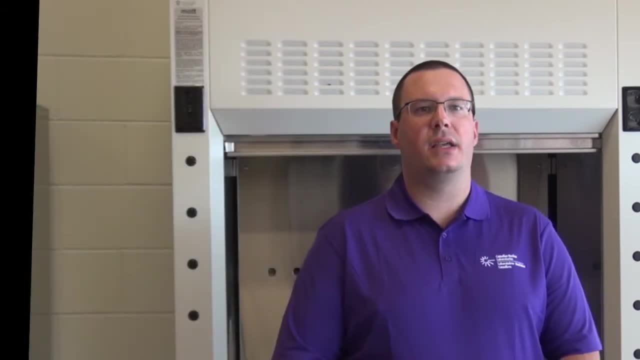 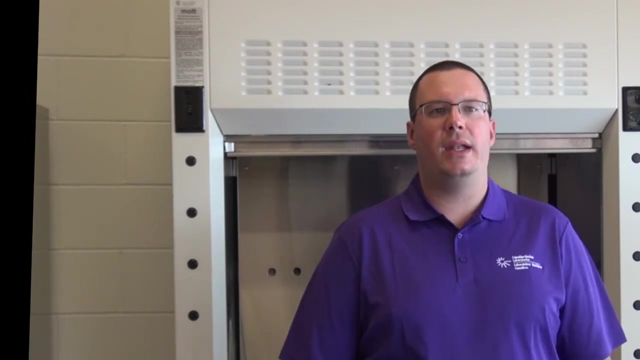 Exposure limitation. In radiation protection, exposure limitation is done largely by applying time, distance and shielding techniques to a task. These type of techniques can be applied to COVID-19 as well, to limit the potential of exposures during the work In the nuclear industry, just like all industries, once hazards and risks are evaluated, plans can be created to reduce the risks to personnel while they work in a hazard area. 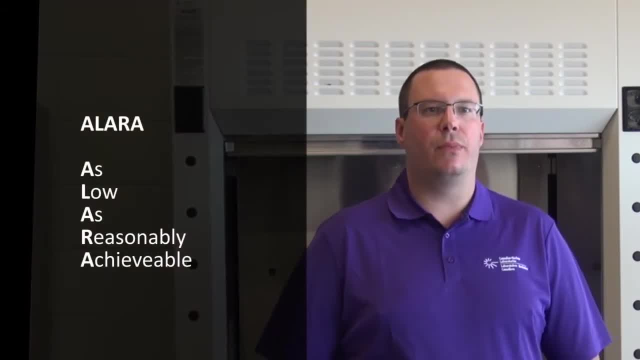 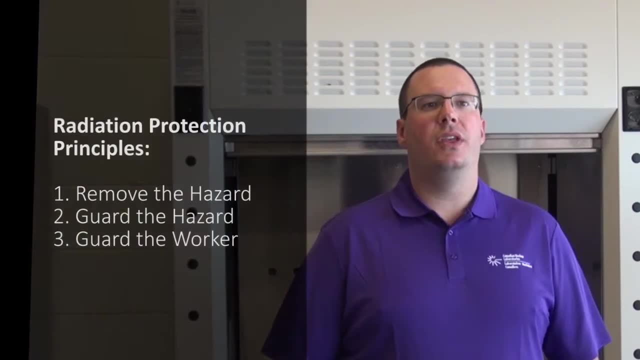 In addition to the ALERA safety principles, we also use our radiation protection principles to reduce the risk an employee is exposed to. The order in which they are stated – remove the hazard, guard the hazard and guard the worker – is the preferred order in which these principles are applied. 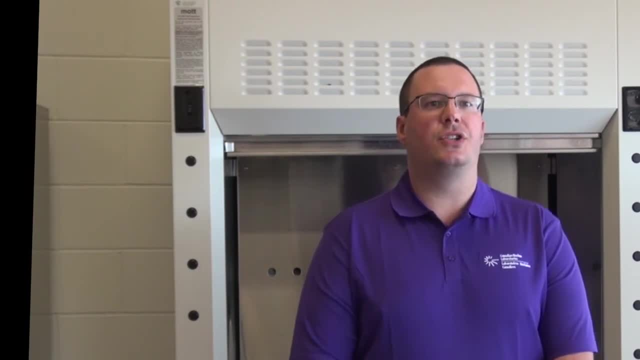 Even if you do not work in the nuclear industry. these practices can be applied at work or at home to reduce your risk. They can even be applied to the things you might do during the pandemic. The first RFP principle we want to look at is remove the hazard. 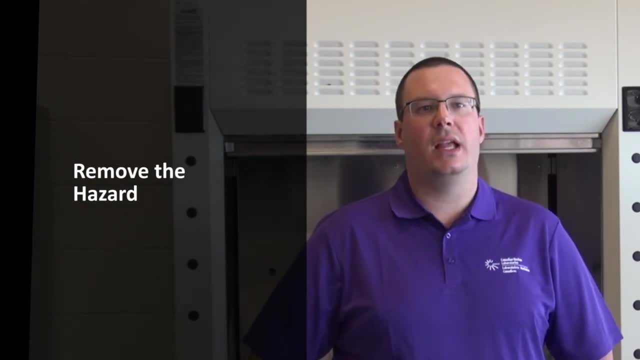 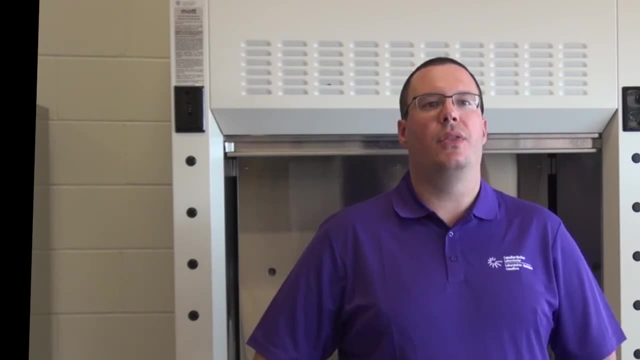 Removing the hazard is always the first thing that will be attempted, as it removes the risk. If the hazard can be removed, the worker is able to complete the job without that exposure. Sometimes, if it is an emergency, the worker is able to complete the job without that exposure. 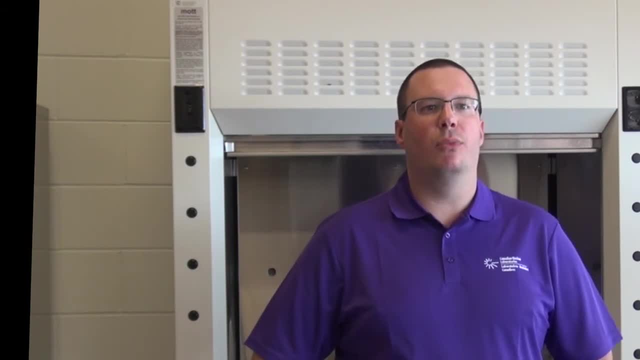 Sometimes, if it is an emergency, the worker is able to complete the job without that exposure. If it is possible that the hazard can be removed completely, the worker can reduce the risk. For us, it is highly recommended to remove theourt radioactive source or clean up contamination before work starts. 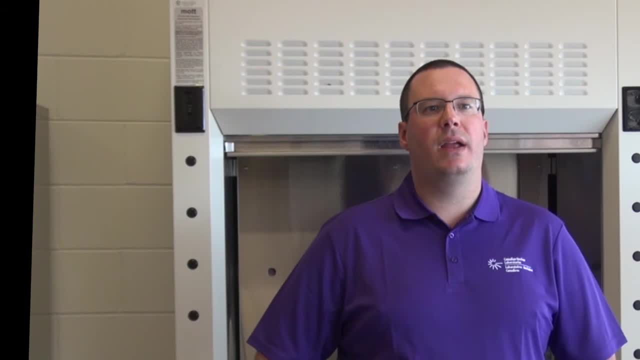 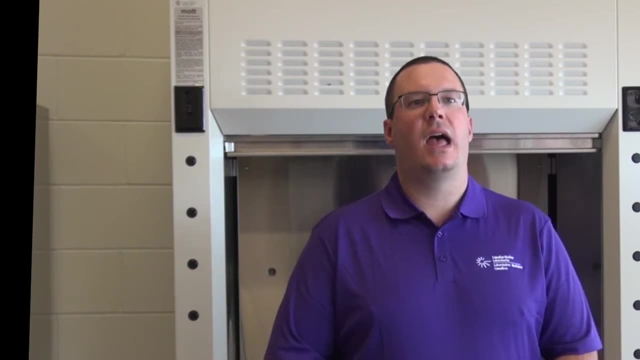 Leaving a patient in change for its treatment In healthcare. this is something like using caretakers who sanitize the room from work to home. At home, this is washing your hands after both hands have been took to the store. If we cannot completely remove the hazard in the nuclear industry, 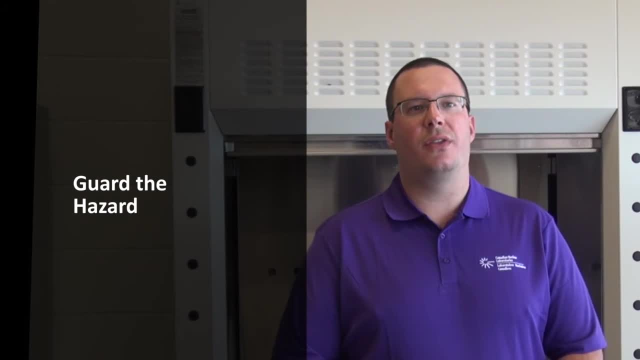 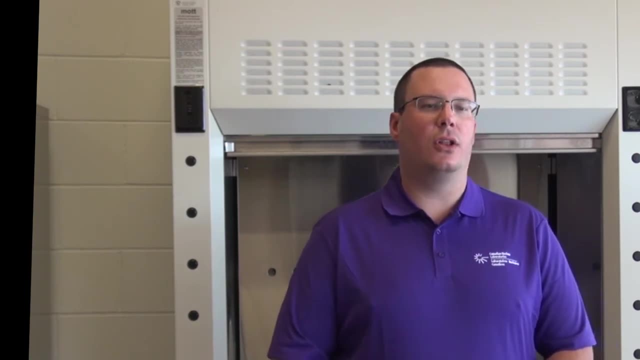 we often use various engineered devices to guard the hazard by keeping it away from the worker. Examples of this are glove boxes, fume hoods and vented enclosures. However, we don't always need to get that fancy. Often we bag, sleeve or cover up a contaminated item so that an individual cannot. 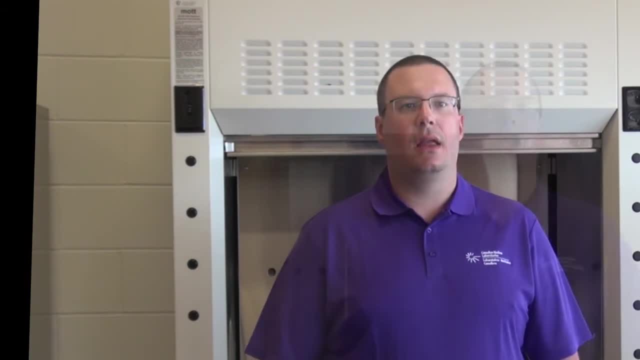 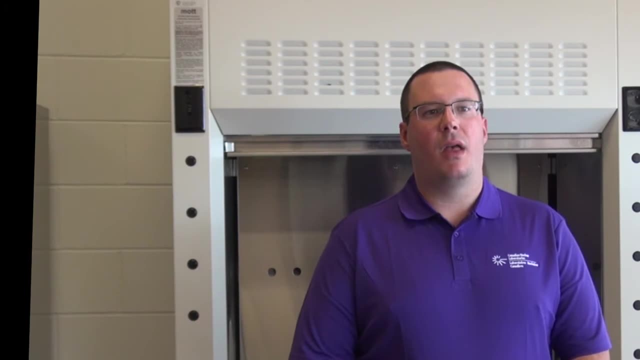 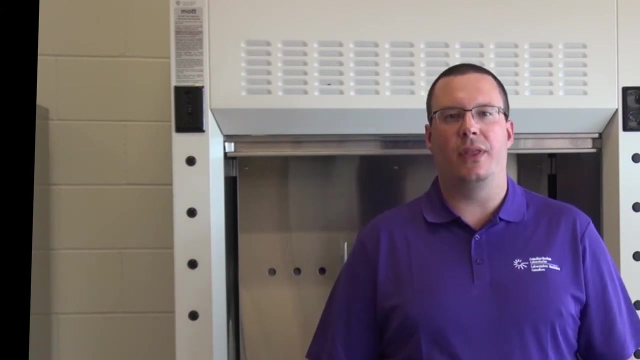 inadvertently come into contact with that by mistake. Examples of this are glove boxes, fume hoods and vented enclosures. However, we don't always need to get that fancy. Often we bag, sleeve or cover a contaminated item so that an individual does not inadvertently come into contact with it. 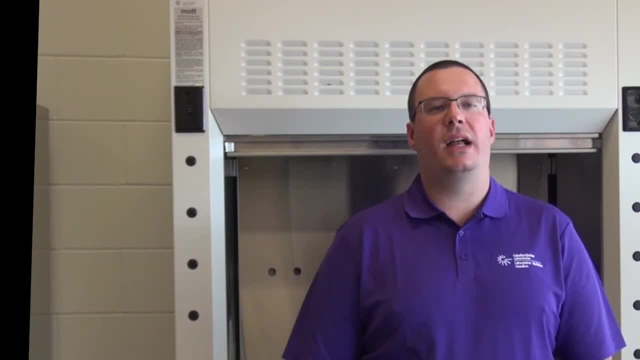 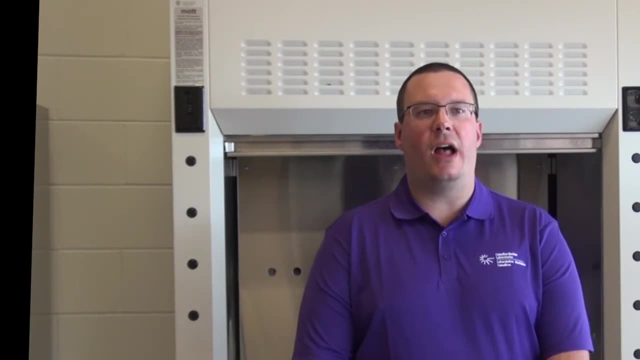 In other industries, guarding the hazard might look like a plexiglass shield for cashiers or curtains between patients in a hospital, or even negative pressure ventilation to help air exchange. If we cannot completely remove the hazard or guard it, then we will guard the worker. 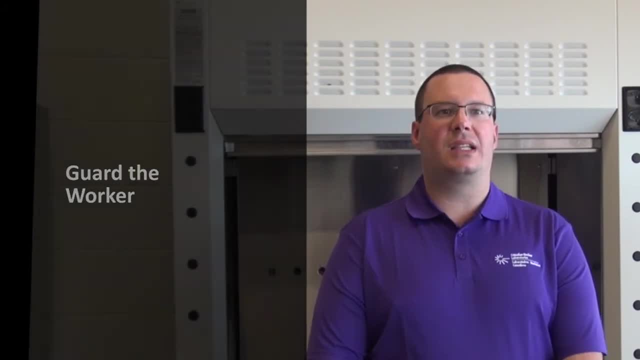 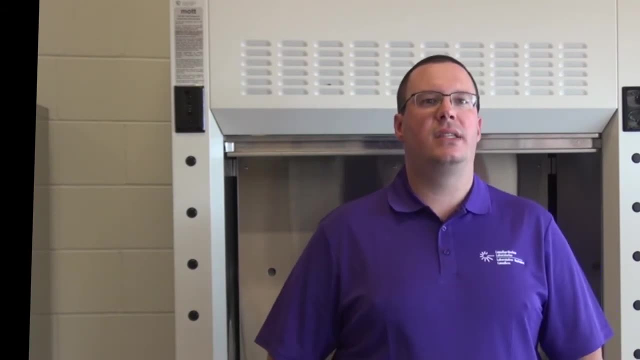 We want the guarding of the worker to always be the last line of defense that we use. Like all industries, we guard the worker by using PPE. This includes things such as goggles and face shields or respirators and rubber gloves. It might also include 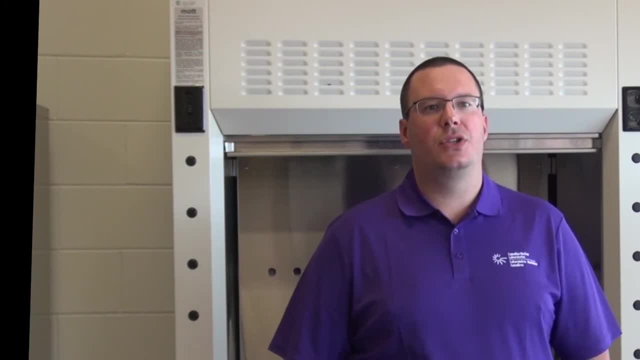 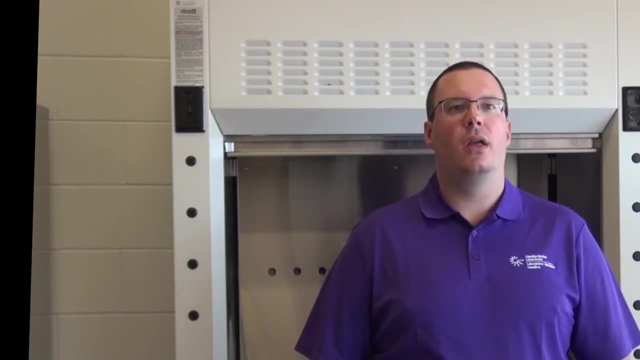 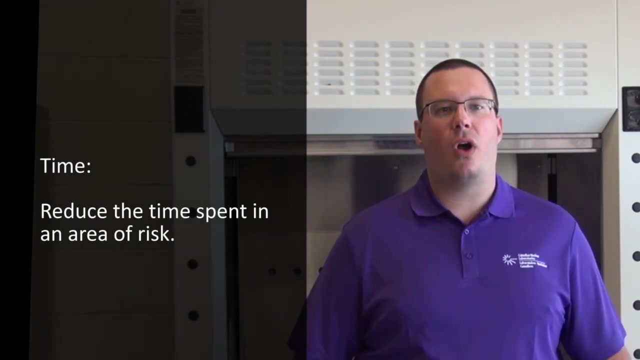 protective suits or gowns. Within the nuclear industry, we also use radiation protection practices such as time, distance and shielding to guard the worker. These can be applied in other industries as well. When looking at time, what we mean is reducing overall time spent in an area of risk. 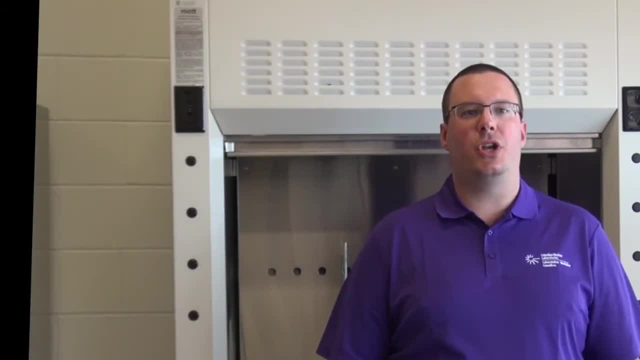 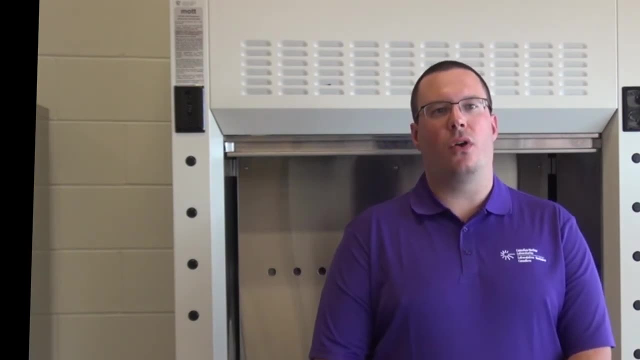 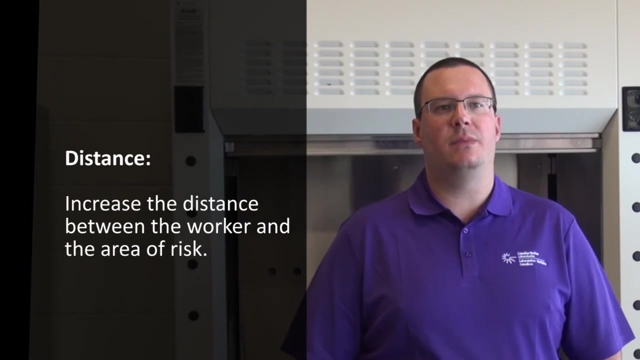 For example, you might cluster your work so that if multiple jobs need to be done in an area of higher risk, you do them all at once. This will reduce the overall time spent in the area and therefore reduce overall exposure For distance. this is increasing the space between the worker and the area of risk. 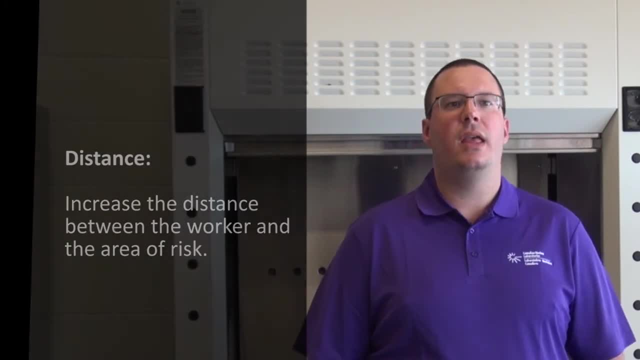 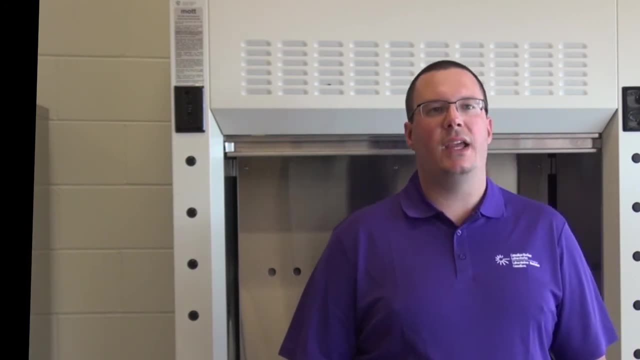 Distance helps to decrease the exposures to radiation in the nuclear industry and works as well with certain biological hazards. For example, we know the recommendation for COVID-19 is to keep two meters apart, thus reducing the risk of spreading the virus. Shielding is exactly what it sounds like. 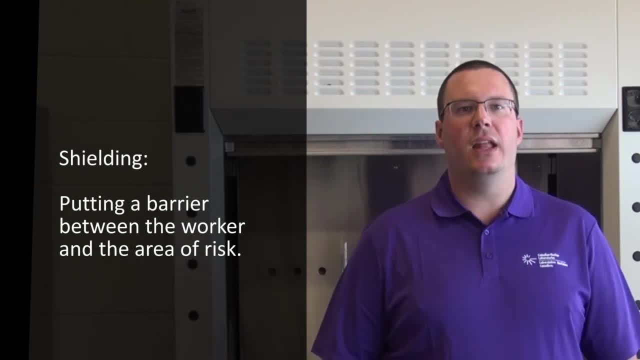 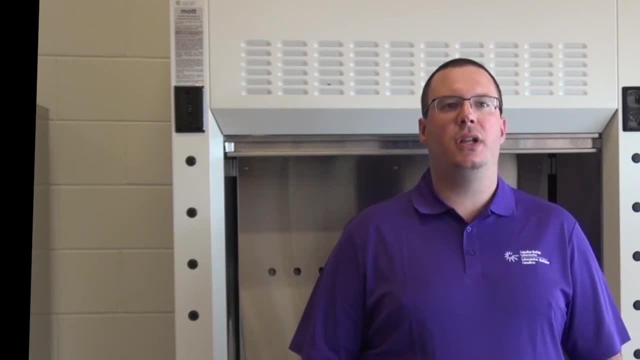 Putting a barrier between the worker and the area of risk. In the nuclear industry using lead shielding helps reduce radiation exposures In healthcare or other jobs. shielding is more like guarding the hazard and can reduce and contain the spread of contaminants In all industries when guarding the worker using PPE. 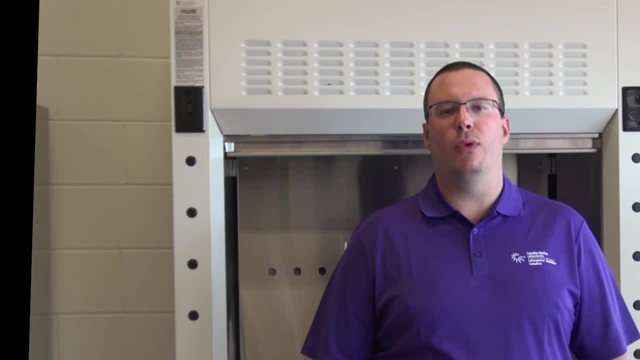 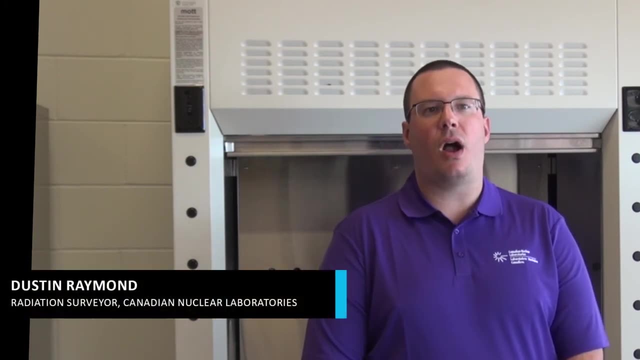 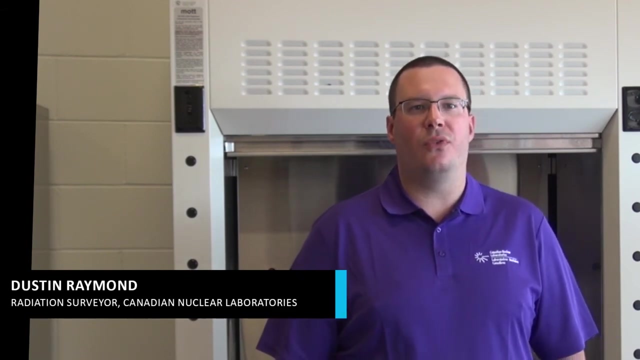 we must remember that is only effective when worn and removed properly. In the nuclear industry we follow procedures to assure that we don and doff PPE properly and safely. But if you are unsure how you should wear PPE, particularly if you haven't had to wear it before, ask the question or find resources to help you. 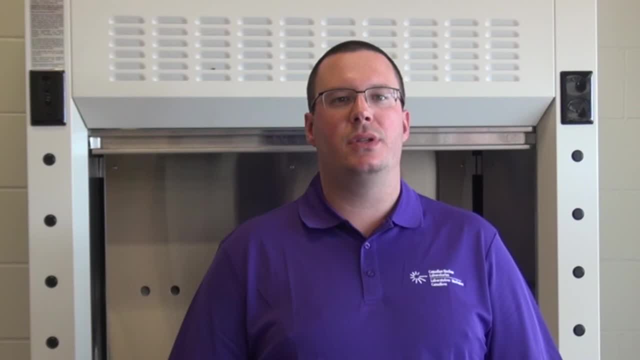 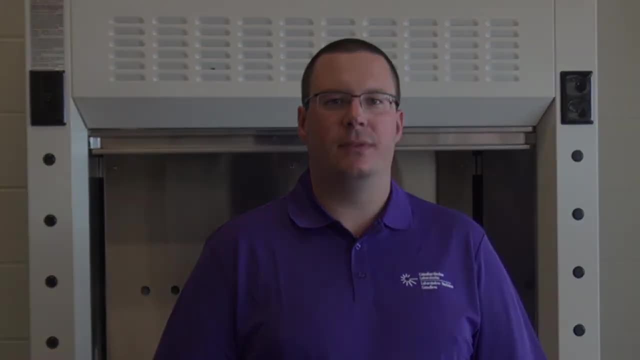 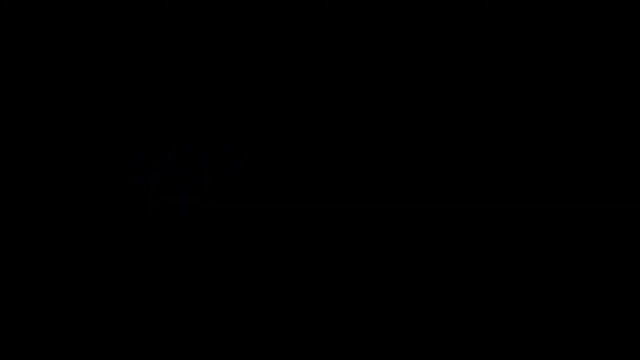 We hope hearing about some of our radiation protection principles can help keep you safe at work and at home. From all of us at CNL, thank you and stay safe you. 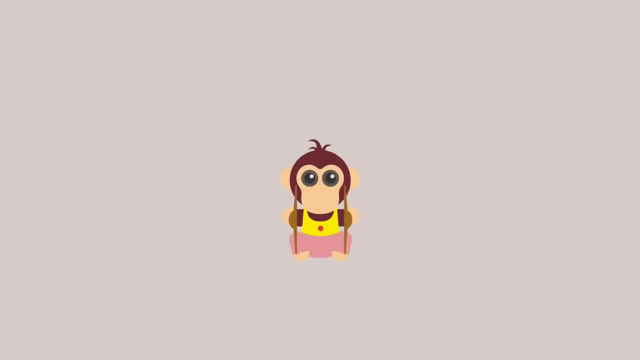 Every piece of music has an underlying beat. A metronome counts out a regular beat. We can speed it up and we can slow it down, but the beats always stay regular. Counting out a beat in fours makes what we call a measure. A measure is just a block of music into which 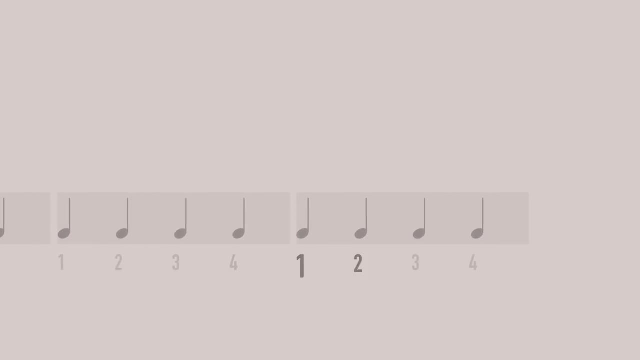 we can drop musical notes. Note symbols show us the rhythm we need to play on top of a beat. Let's listen to these four symbols, one by one, and see what they do. First we have the whole note. A whole note takes up a whole measure, leaving no room for. 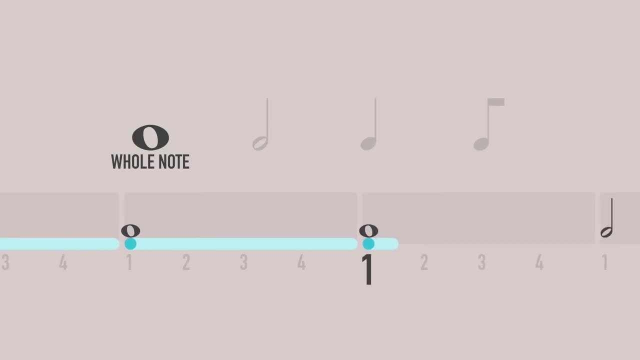 anything else. This means it lasts for four beats. A half note takes up half a measure. This means it lasts only two beats. A quarter note takes only a quarter measure and lasts for one beat. And an eighth note takes up an eighth of a measure and lasts only half a beat. This makes 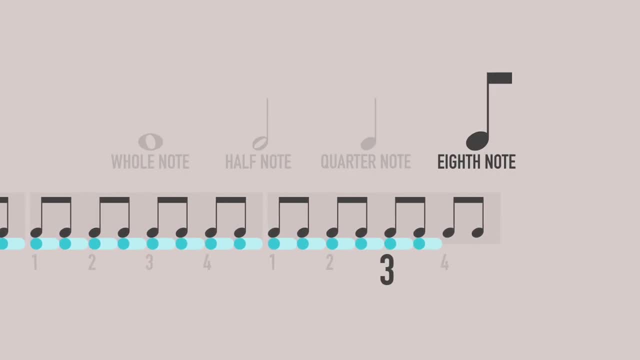 the eighth note a little more tricky because it's faster and we have to count it differently. When we count 1,, 2,, 3,, 4,, 5,, 6,, 7,, 8,, 9,, 10,, 11,, 12,, 13,, 14,, 15,, 16,, 17,, 18,, 19,, 20,, 21,, 22,.